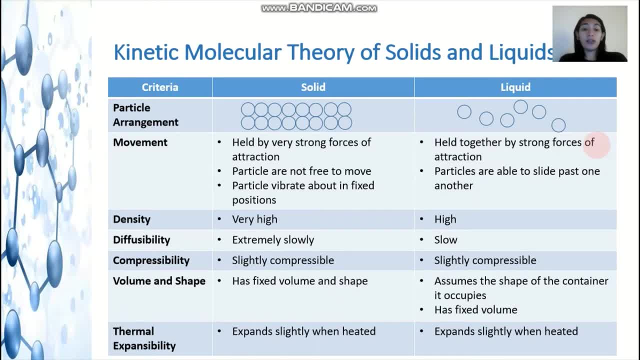 So solid has a fixed volume and shape and your liquid assumes the shape of the container it occupies and it has fixed volume. Now in kinetic molecular theory we also relate its thermal expansions. So it expands slightly when heated, for the solids, while it expands. 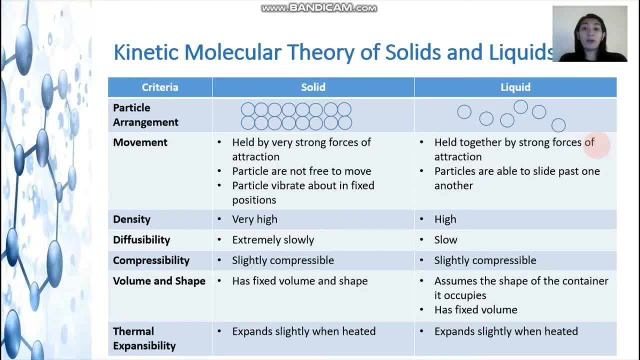 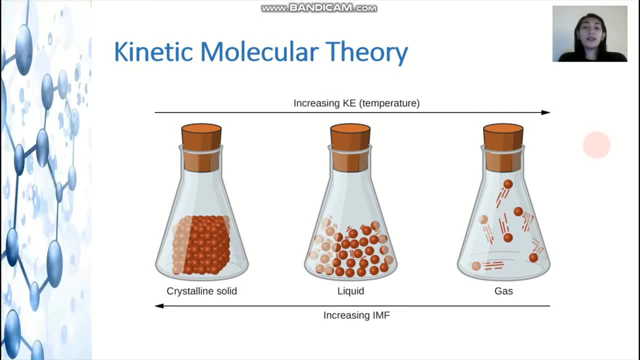 it also expands slightly when heated for the liquid, So the expansion is light because of heat. okay, So the kinetic molecular theory, or the KMT, actually states that when you increase the kinetic energy or the temperature, there's actually a decrease in the intermolecular forces. okay, 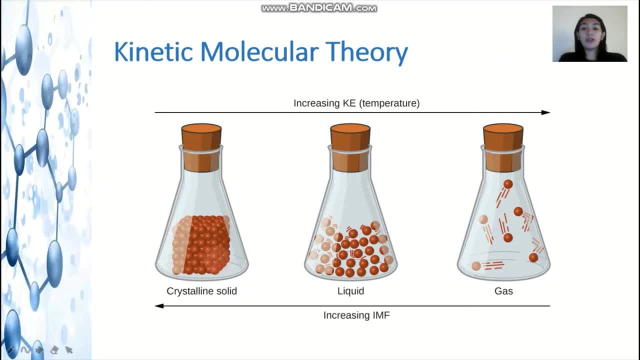 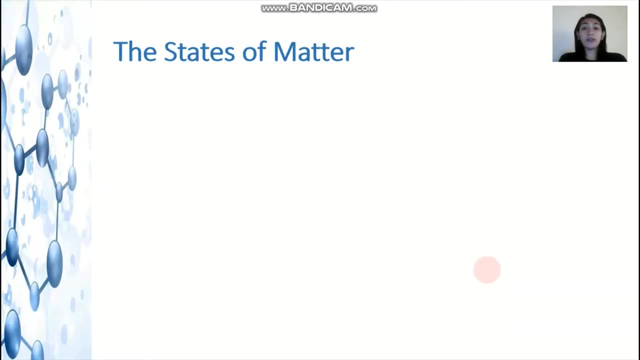 So for the solids, as you can see, the molecules are compact, so liquids are slightly moving, while for the gases, the molecules are freely moving. okay, Now what are intermolecular forces? So that would be the highlight of our video. 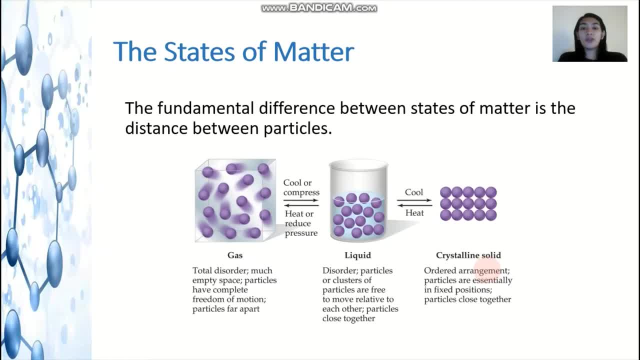 Now let's just have a recap of the states of matter. So, as you could see, the fundamental difference between the states of matter is actually the distance between the particles. So now that you are in the in senior high school, you should not just differentiate the states of matter by its different characteristics. 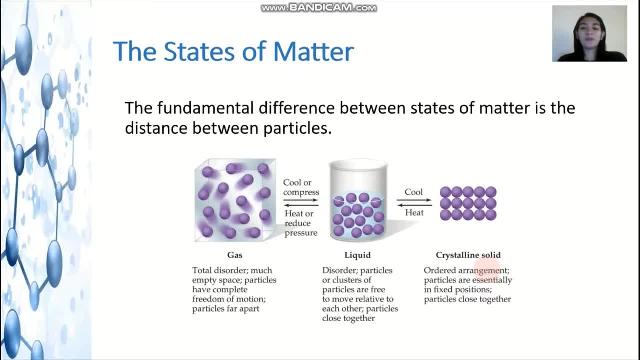 So you need to. this is the more advanced description or differentiation of the states of matter. okay, So for gases there is total disorder and there's much empty space, while for the liquid, minimum disorder and the particles are, clusters of particles are free to move. 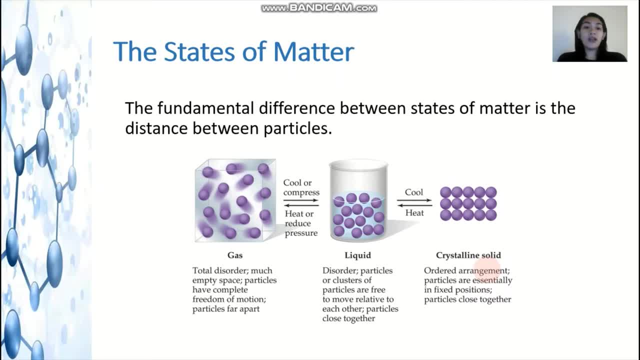 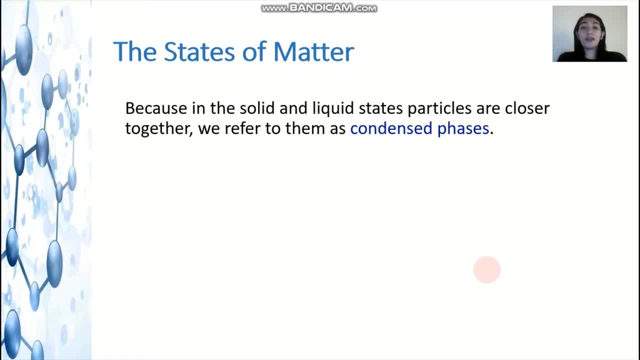 relative to each other. okay, So for the solids, there is the ordered arrangement of your particles. okay Now, because in the solid and liquid states particles are closer together. we refer to them as the condensed phases. The state of a substance is in that the particular temperature and pressure depends on two antagonistic entities. 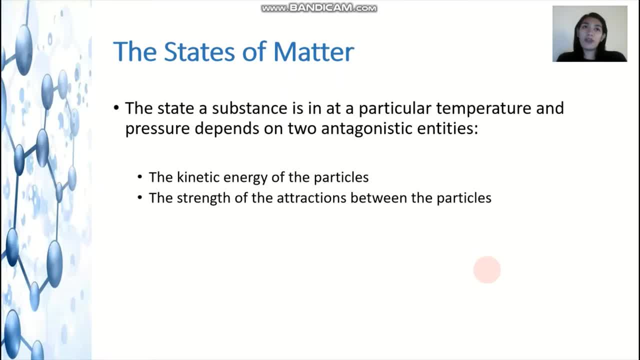 So one is the kinetic energy of the particles. So we define your kinetic energy as So we define your kinetic energy as. So we define your kinetic energy, as is the energy in motion, and also we have the strength of the attractions between the particles. 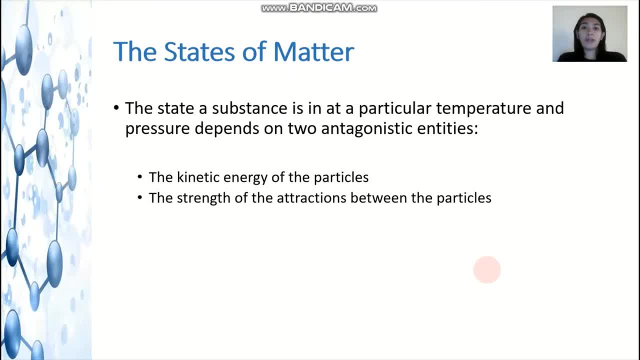 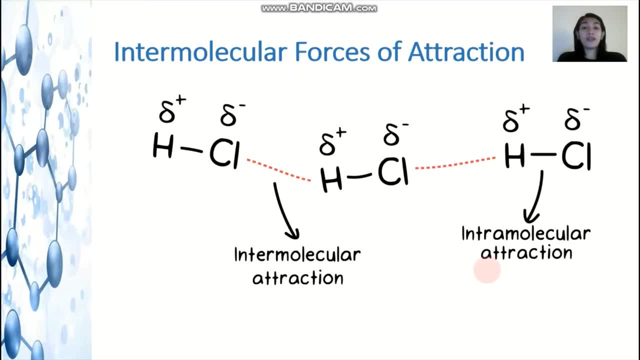 okay, so yung attraction, yun yung ating pag-uusapin in this video today. okay now, we have now two types of forces of attraction. you have the intermolecular attraction and the intramolecular attraction. okay, so, here in the intermolecular, so you have two. 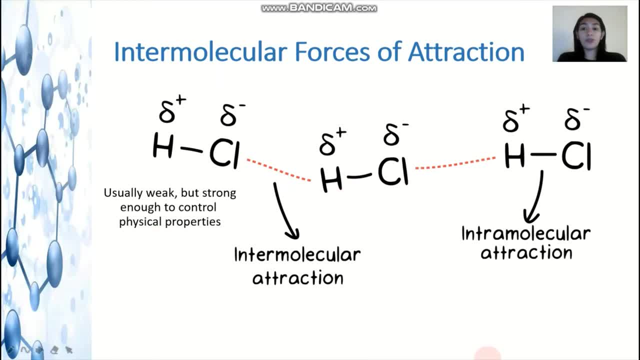 molecules, two different molecules, so usually they are weak but strong enough to control your physical properties. while for the intramolecular attraction, these are the force which keeps the molecules together. this one, so it's similar to your bonding. okay, so the intermolecular attraction is also the attractive force between your molecules, so it is responsible for keeping 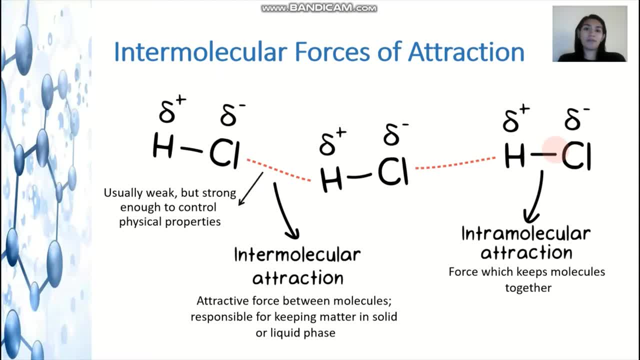 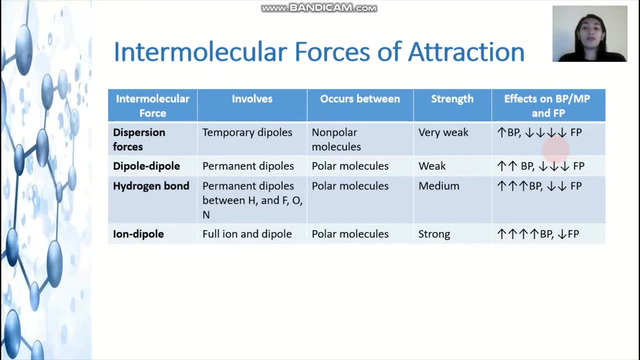 matter in solid or in liquid phase. okay, now these are the basic types of the intermolecular forces of attraction. so first we have the dispersion forces, so it actually involves temporary dipoles. okay, when we talk about dipoles, it refers now to the separation of the charges of your molecules. okay, so later on. 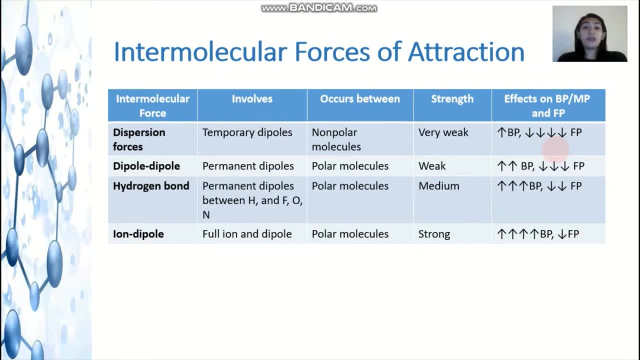 in your in in the next slide- next slides- you would see the an image of your dipoles. okay, so this table summarizes the different types. let's just have an overview. so for the dispersion forces, they occur between non-polar molecules and they're very weak. okay, so when you increase the boiling point, there would be a decrease in the. 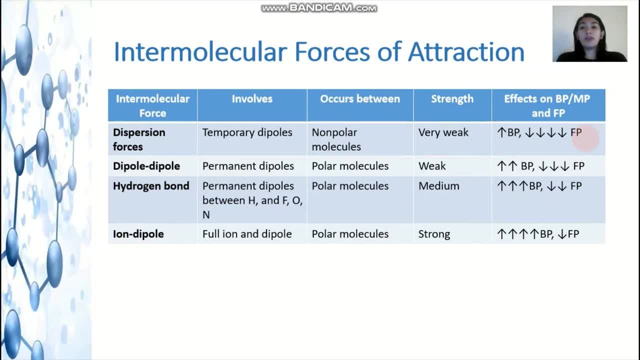 freezing point. okay. now dipole, dipole, molecular force are happening in permanent dipoles and they occur in polar molecules. so they are weak forces. okay. so if you have a dispersion force and you have a dipole, dipole molecular force, it is just a weak attraction. let's just have the effects of 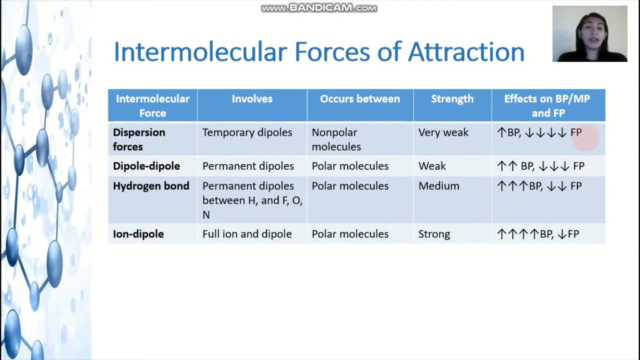 the bp refers to the boiling point, mp refers to the melting point and fp refers to the freezing point. okay, so later now let's just go through it. okay now. hydrogen bond. so these are permanent dipoles between hydrogen and fluorine, oxygen and nitrogen. so it happens in your polar molecules and the 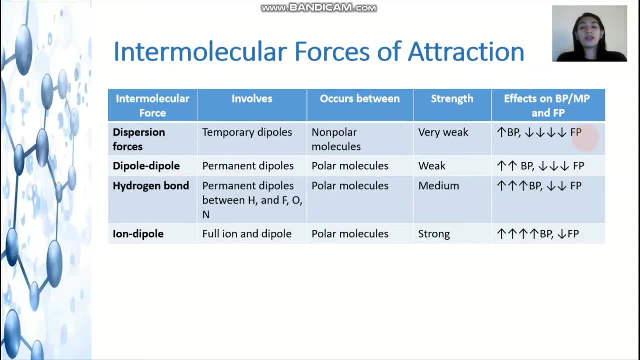 strength is at the medium level. well, the strongest among the intermolecular forces is the ion dipole force of attraction. so it happens in a full ion and dipole. so what is an ion? so recap, so these are your charged um elements. okay, so this happened. this um attraction happens in your polar molecules. 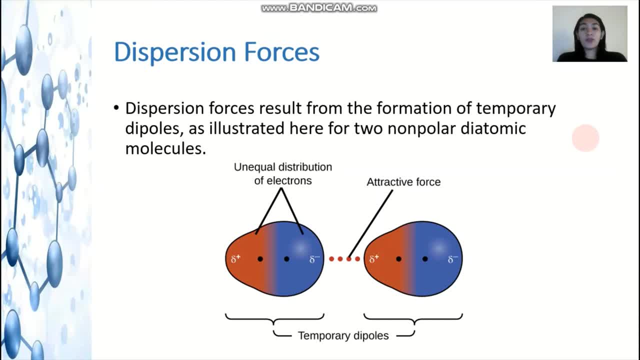 okay, let's go to your dispersion forces. so this actually results from the formation of temporary dipoles, as illustrated here. you have two non-polar diatomic molecules. so you see, at the shahian asinusabi natin. so this is the dipole moment. okay, so there's an equal distribution of the. 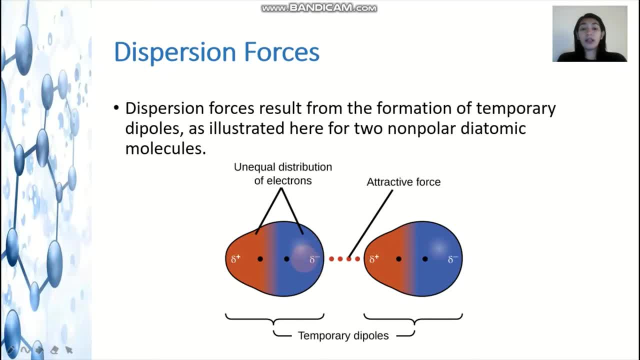 electrons. so you see, here these are the positively- i'm sorry, negative, partially negatively charged, and you have here the partially positive, your symbol that represents partial, okay, partial positive and partial negative, and you see now a very weak, um attractive force yet. so it is also known as the london dispersion forces. so these are attractions between your. 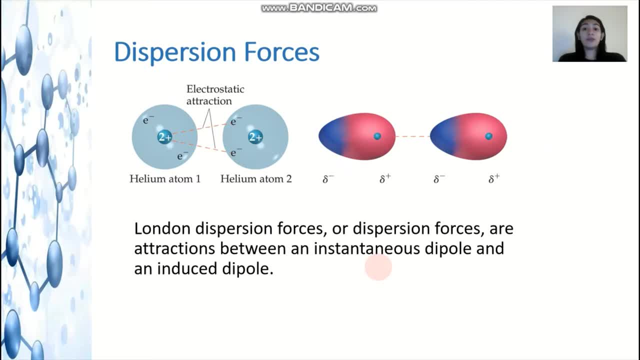 instantaneous dipole and an induced dipoles. so when we say instantaneous dipole, it means it is a dipole at the moment, while an induce dipole is triggered to be dipole for the attraction- okay. for the for the attraction to happen, okay. so these forces are present in all molecules, whether they are positive or negative. 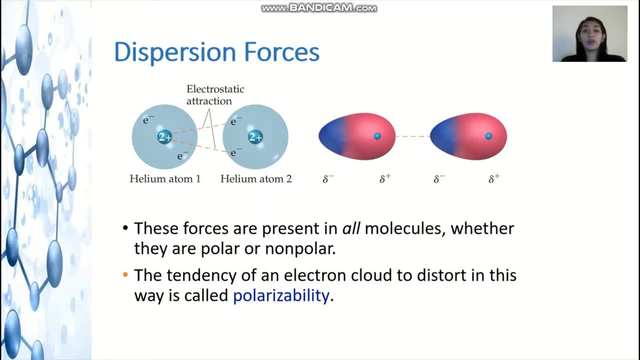 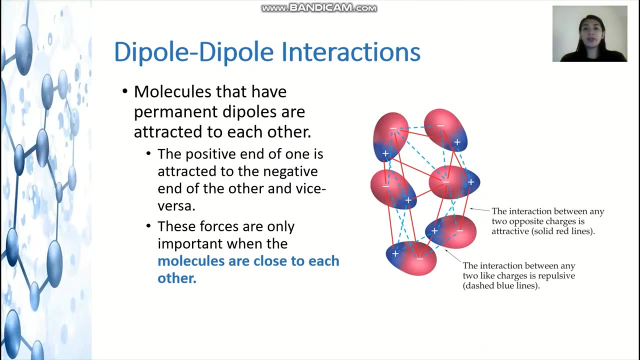 or nonpolar, and the tendency of an electron cloud to distort, as you can see, but there is some a different difference in the shape. the tendency of an electron cloud to distort in this way is called polarizability. so next we have dipole dipole interaction. so this happens when your molecules that are permanent dipoles 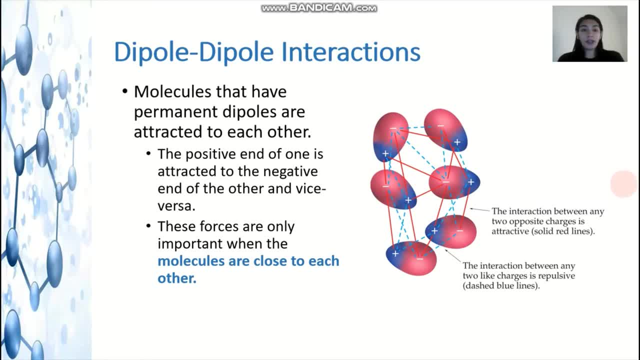 are attracted to each other. so in this picture you see here you have solid red line. so this represents of the interaction between any two opposite charges. well, this one would represent the dashed blue lines represent the repulsive charges. okay, so the positive and the one is attracted to the negative. 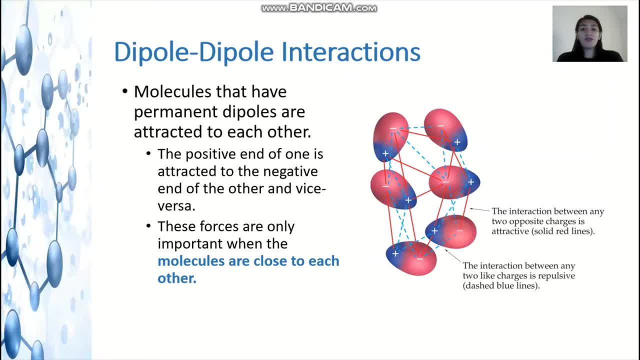 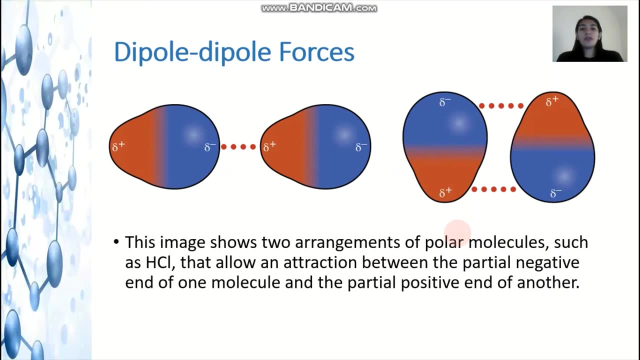 end of the other end, vice versa. so these forces are only important when the molecules are close to each other. so when you increase the distance, there will be much less interaction. okay so, Yann? so in this image you see two arrangements of the polar molecules, such as your hydrochloric acid. so 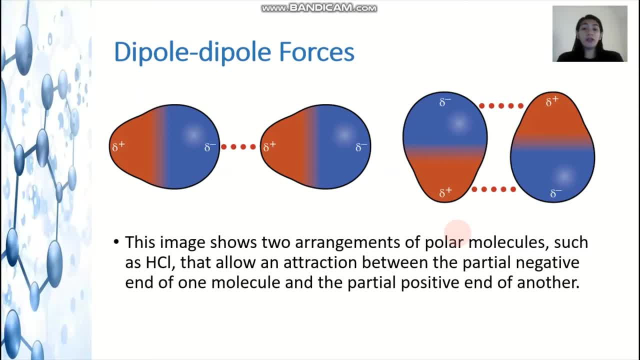 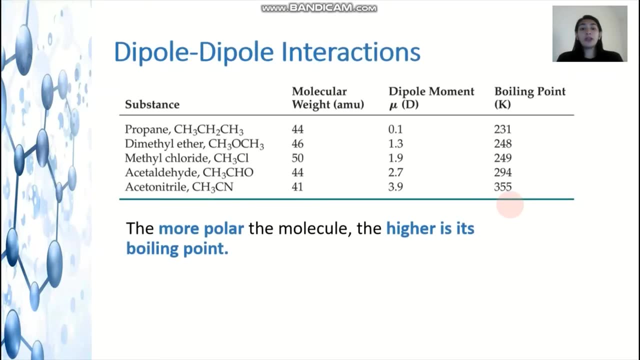 it allows an attraction between the partial negative end of one molecule and the partial positive end of the other. okay, so it could be done at this way, or the opposite. okay, so for dipole-dipole interactions, the more polar the molecule, the higher is its boiling point. okay. 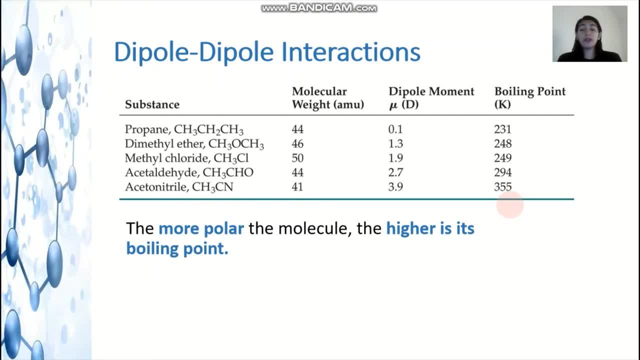 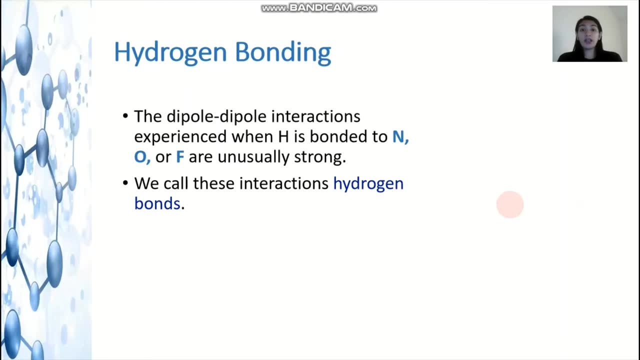 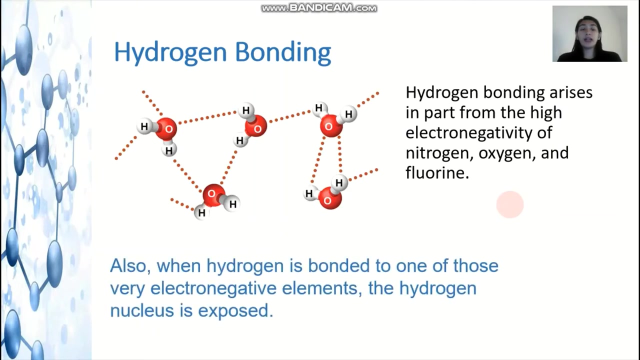 so here are some examples of your substances or molecules, or i mean compounds. so yeah, now hydrogen bonding, as mentioned, and bonding of hydrogen to nitrogen oxygen and chlorine. okay, so we call these interactions hydrogen, simply your hydrogen bonds. so hydrogen bonding arises in part from the high electronegativity of these elements: nitrogen oxygen and fluorine. okay, so also when hydrogen, 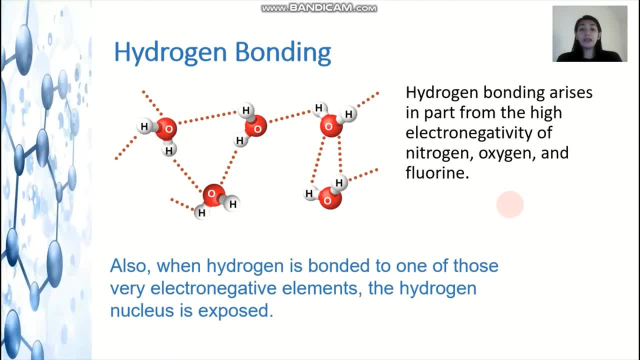 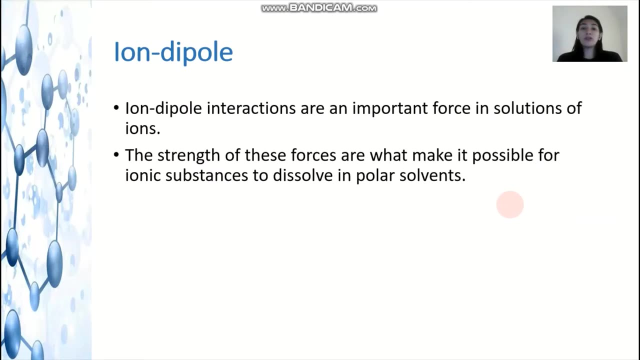 responded to one of these very electronegatives. the element, i mean the hydrogen nucleus, is actually exposed because the electrons are bonded. okay, so last we have the ion dipole charge, i mean, i'm sorry, the ion dipole interaction. so this is um an important force and solutions of ions, okay. 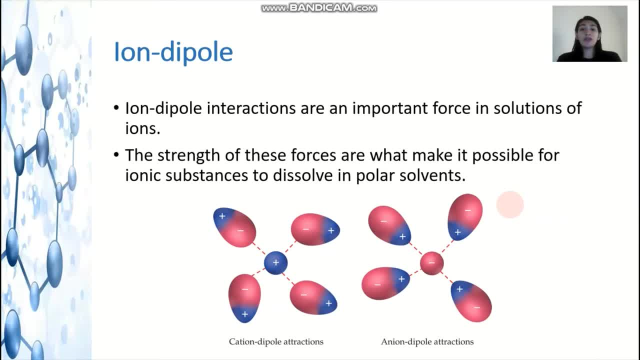 so the strength of these forces are what makes it possible for ionic substances to dissolve in polar solvents. okay, so you have here the cation dipole attraction, so cation is in the center, while the other one we have the anion dipole attraction. so, as you can see, um there are. these are the partially positive side attracted. 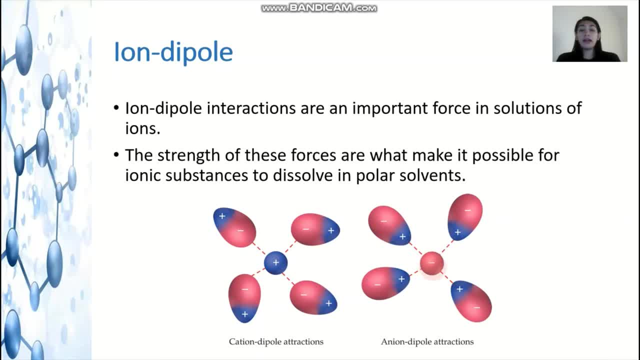 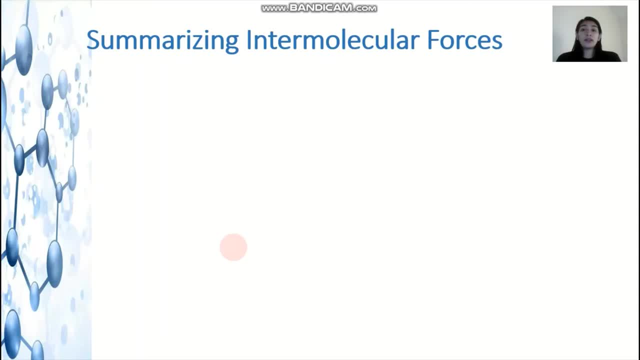 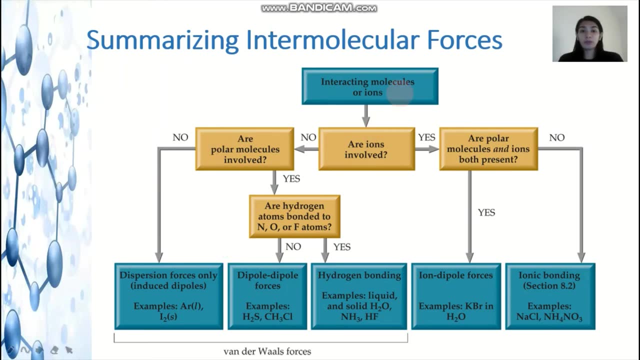 to the very strong attraction of the anion. so same with our cation. okay, so for you to further analyze your intermolecular forces, you may ask yourself this following question: okay, so follow the flow chart. so do you have interacting molecules or ions? so are ions. 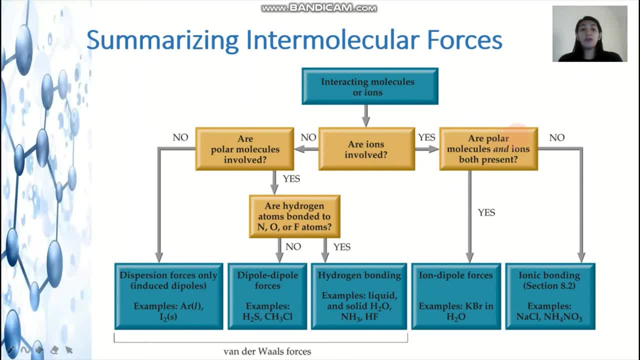 involved? if yes, ask yourself: are polar molecules and ions will present? if yes, then it is an ion dipole force, but if it's not, so it is an ionic bonding. so let's, we'll have a separate lecture on that. so if ions are not involved, we ask our polar molecules involved? so if yes, you ask yourself: 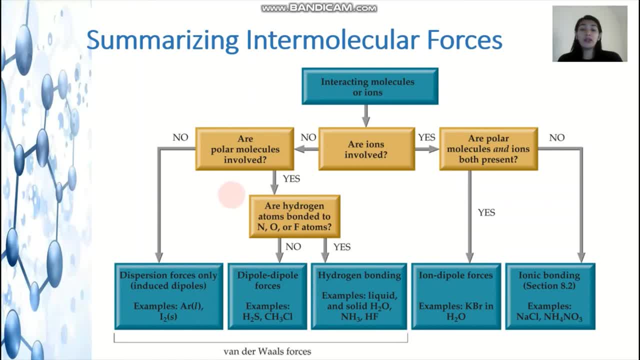 are hydrogen atoms bonded to nitrogen, oxygen and fluorine. so if if no, it is a dipole dipole force. but if yes, it is simply your hydrogen bonding, okay. so if no poly molecules are involved, then these are simply your dispersion forces, or the induced dipoles, okay. so now let's go to the 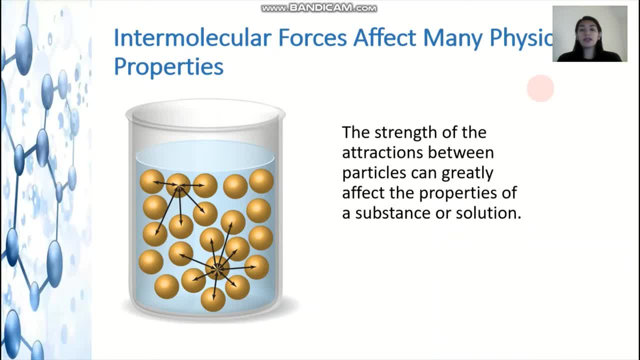 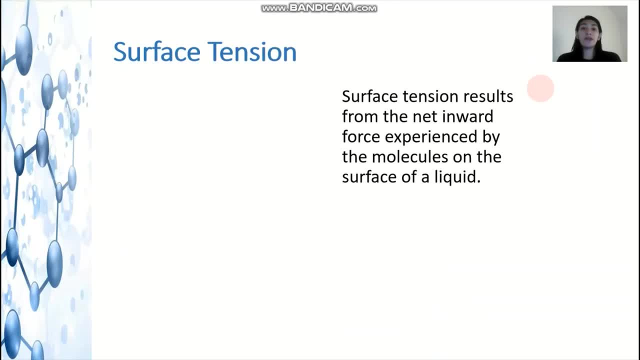 physical properties affected by the intermolecular forces. okay, so the strength of the attractions between particles can greatly affect the properties of a substance or solution. okay, so first we have your surface tension. so surface tension actually results from the net inward force experienced by the molecules on the surface of a liquid. okay, so another is viscosity. so 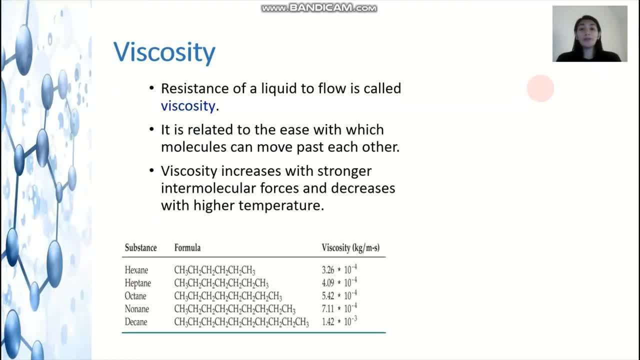 viscosity refers to the resistance of a liquid to flow, and it's related to the ease with each with which molecules can move past is on past each other. okay, so viscosity actually increases with stronger intermolecular forces. so this is the resistance of a liquid to flow. 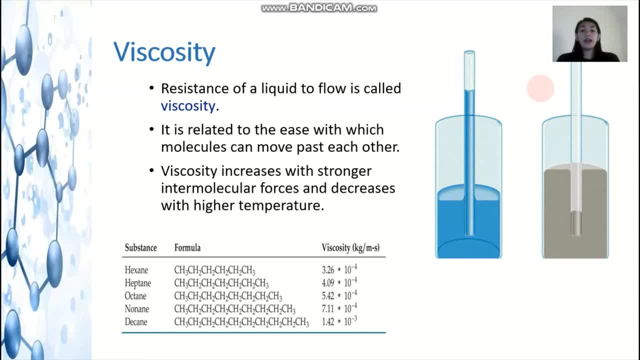 intermolecular forces and it decreases with higher temperature. okay, so yeah, you could see now adhesion versus cohesion. so adhesion is the attraction between, unlike molecules. so, as you could see, here the liquid is attracted to glass. well, for here you have cohesion, it is the 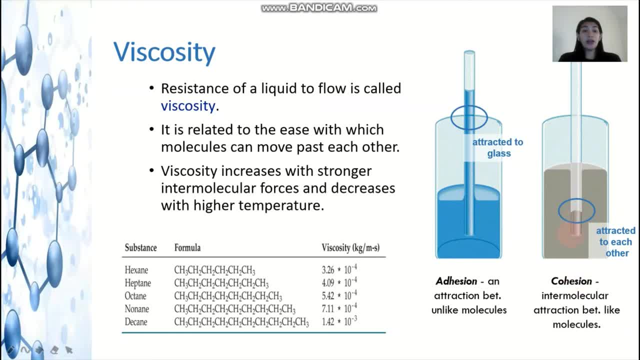 intermolecular attraction between like molecules. so here you would see now the attraction of the liquid to each, to each other. okay, so adhesion is in thatо when mol is attracted to glass, the water is driven by the adhesion. when mol is attracted to glass, it can become adhesive, it can become more resistant to water. 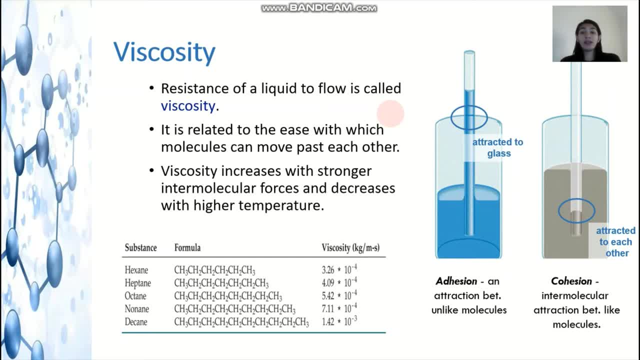 okay. and if it is not attracted to water, it is because of adhesion, while here that they get together, it's because of cohesion, can you realize? okay, so once these molecules are attracted- now i mean to the glass, it can be adhered. okay, so you have adhesion. okay, so viscosity: 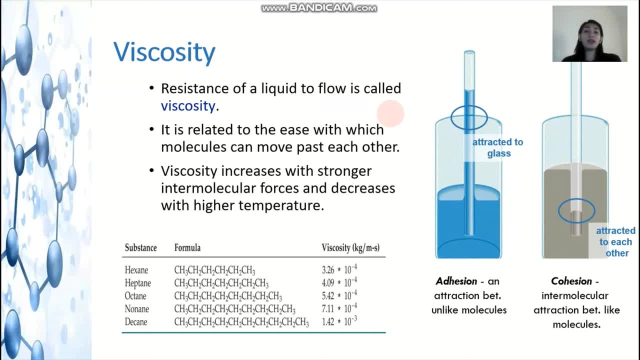 we said resistance of a liquid to flow. so when you decrease, it decreases with higher temperature. so that means it is easier to do that now. it is easier to absorb. or you can put that on a mag flow ngayon yung liquid pag mas mataas ang temperature. okay, we also have your vapor pressure. 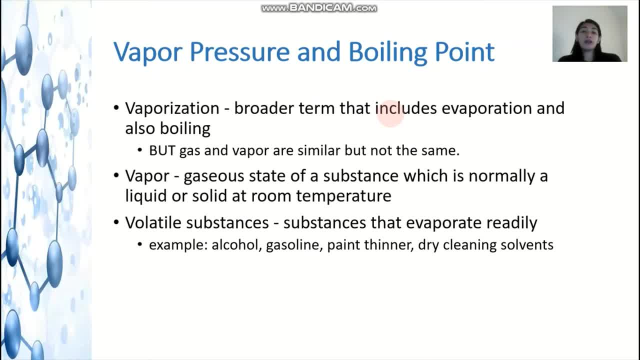 and boiling point. so vaporization is actually a broader term that includes evaporation and also boiling. okay, so you may think that gas and vapor are the same, but actually they're not. so they're just similar because yung vapor is actually a gaseous state of a substance which is normally 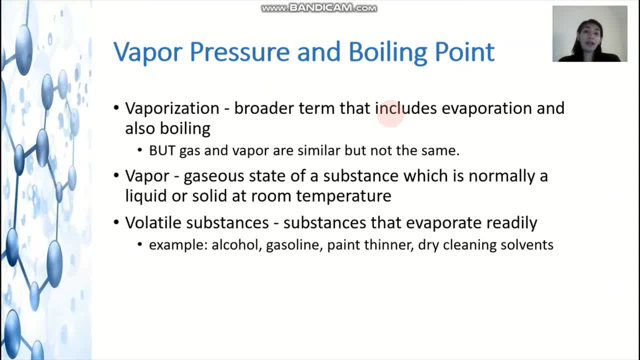 a liquid or solid at room temperature, while yung gas it is the state of matter. okay, so the volatile substances are substances that evaporate readily, example yung alcohol, gasoline, paint thinner and dry cleaning solvents. okay, try nyong mag iwan ng bottle of alcohol open. 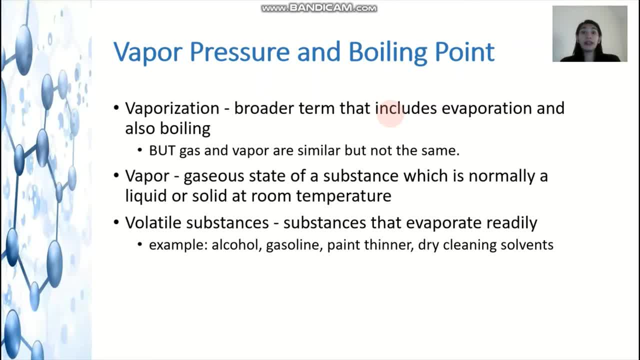 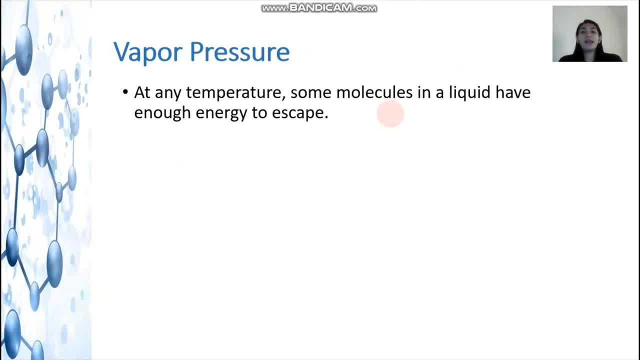 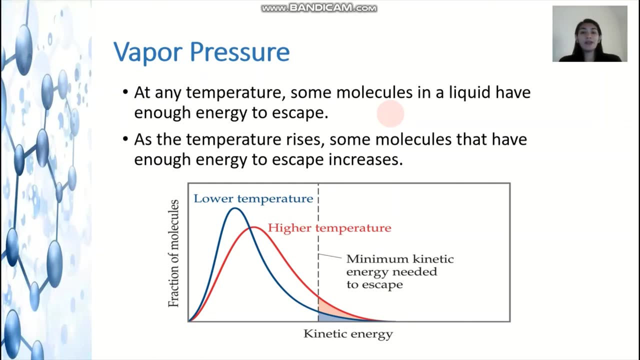 siguro iwan nyo sya for a week. makita nyo na nag decrease yung ano nya a month. okay. so yun ang madali sya mag evaporate. okay, vapor pressure. so at any temperature some molecules in a liquid have enough energy to escape. okay. so as the temperature 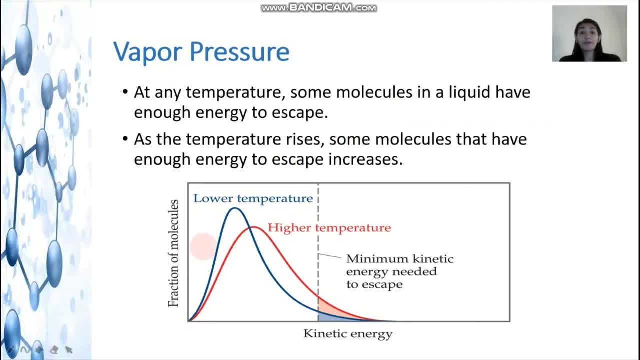 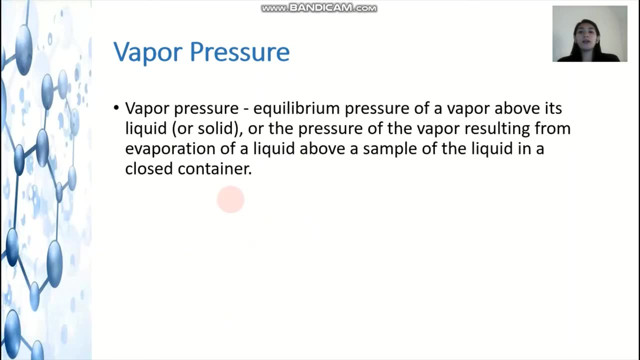 rises, some molecules that have enough energy to escape actually increases. so here, as you see, when there is an increase in kinetic energy and some of the molecules would be actually moving out. okay, so the vapor pressure is actually the equilibrium pressure of a vapor above its liquid or solid. 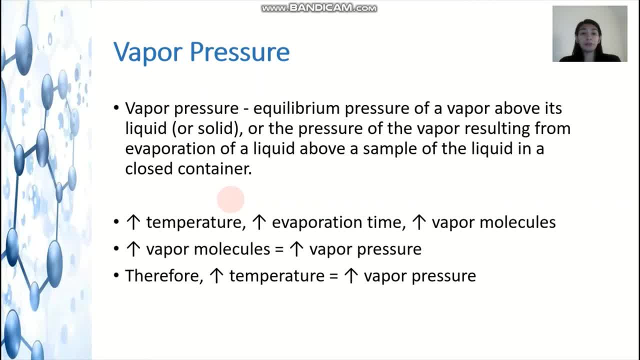 okay. or the pressure of the vapor resulting from evaporation of a liquid above a sample of the liquid in a closed container. so once you increase the temperature, there is an increase in evaporation time and there is also the increase in vapor molecules. now, if there is an increase in the 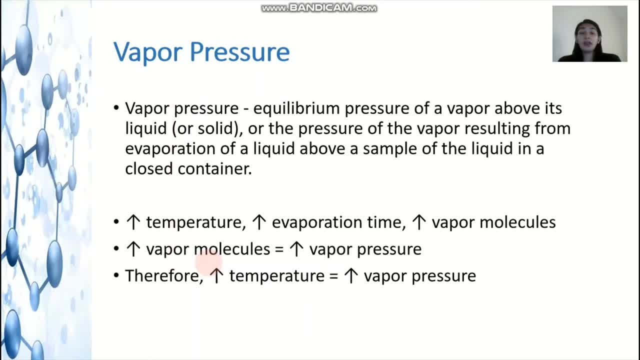 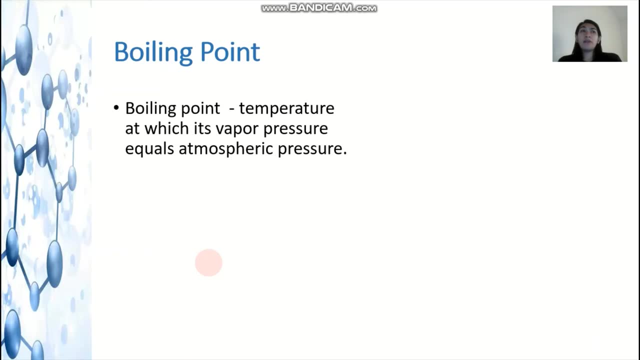 vapor molecules there would be, it would equate to the increase also of your vapor pressure. therefore, an increase in temperature would be also and it would mean an increase in vapor pressure. okay, so next we have a boiling point. so when we boil water, if we see that at 100 degrees, 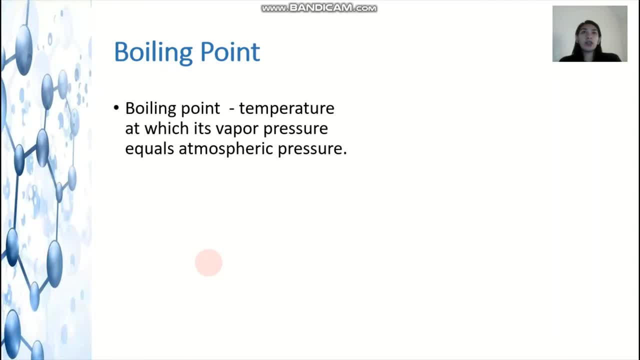 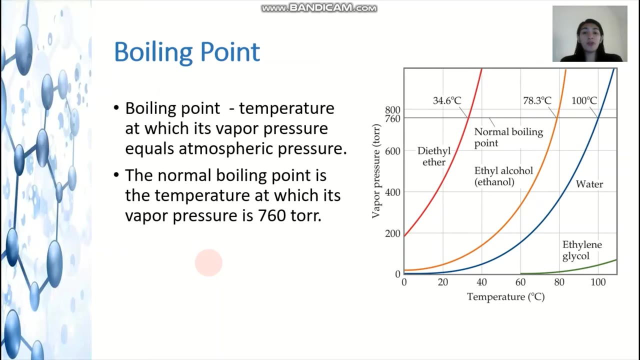 we don't have a thermometer. we know that the water is boiling, because that is the property of water. okay, so the boiling point is a temperature at which its vapor pressure equals the atmospheric pressure. so the normal boiling point is a temperature at which its vapor pressure is 760. 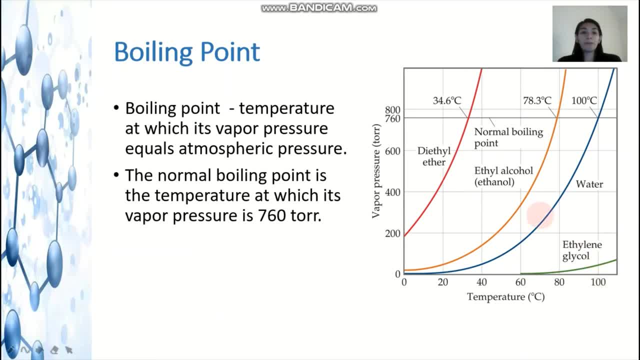 or okay. so on the right, you have now um the different boiling temperatures, or i mean boiling point of different um liquids. so we have here the diethyl ether, then you have your ethyl alcohol and your water. okay, so when you combine ethanol and water, usually the wine or the alcoholic 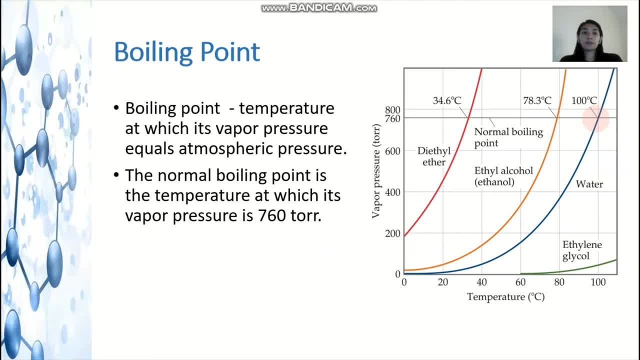 beverages. try to boil them. you will see that they are boiling first. after evaporation, the alcohol will dissolve or the alcohol will boil. okay, so since alcohol is volatile, it is easier to vaporize then, because at 78.3 degrees celsius it has already boiled. 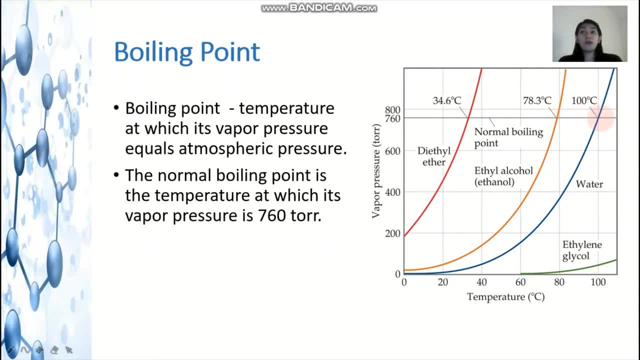 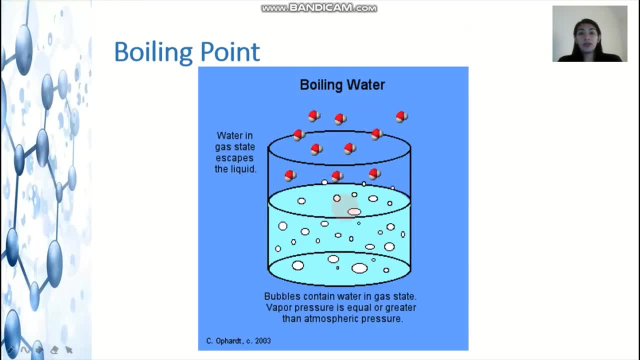 so if you increase it it will just remain the water content of the alcohol. okay, so there you see. so in the boiling point we have the water content of the alcohol and then we have the vaporized alcohol. at this point water and gas state actually escapes in the liquid. okay, so here the bubbles contain. 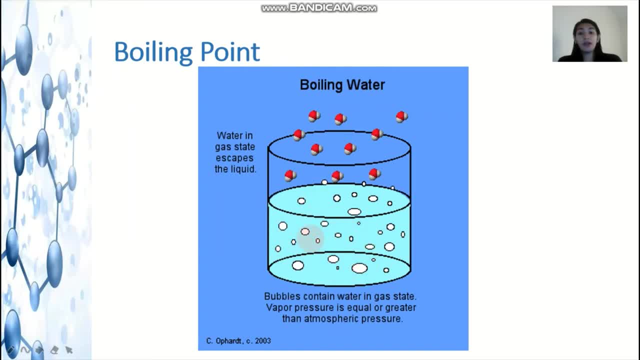 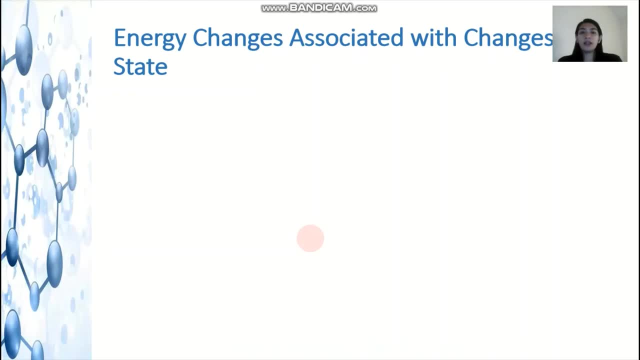 water in the gas state. okay, at this point vapor pressure is equal than or greater than the atmospheric pressure. okay, now let's just have an overview of the energy changes associated with changes of state. so we have the heat of vaporization, or this is the amount of heat needed. 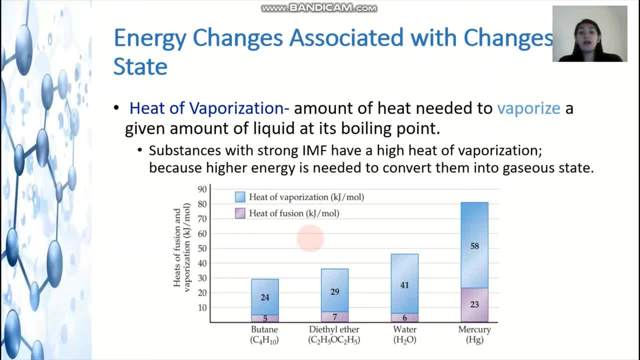 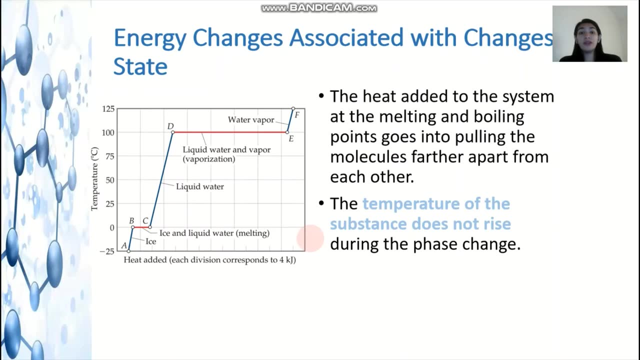 to vaporize a given amount of liquid at its boiling point. okay, so substances with strong intermolecular force of a high heat of vaporization, because we need higher energy to convert them into a gaseous state. next, we have not, not yet the next one. 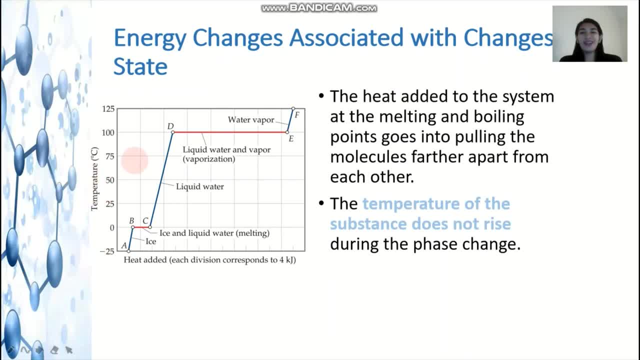 so here we actually have a graph that actually tells us the heat of vaporization. okay, so the heat added to the system, so you would see here the changes in the phases. okay, so, for example, here it is at the A to B- solid, so it's ice. then it starts to melt, so ice and 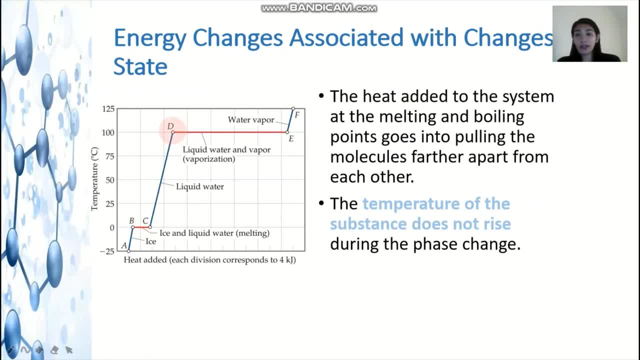 liquid water here. then you have here this phase and the 100 degrees Celsius. again water in a shot, it's at the rock. a mama and I am. another discussion on this. okay, now the heat added to the system at the melting and boiling point points go into, goes into pulling the molecules further apart from each other's again. 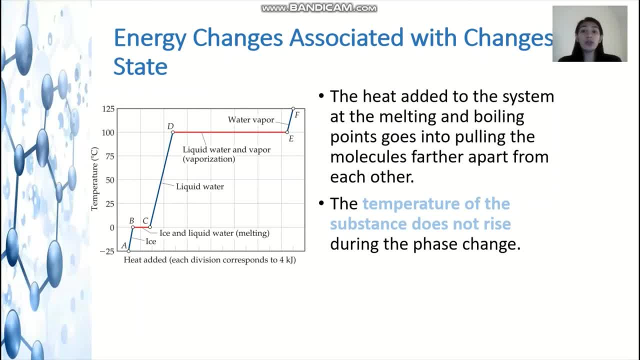 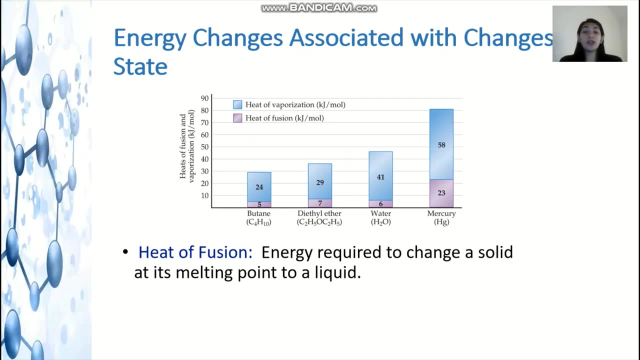 kinetic molecular theory. so as you increase the temperature there's an increase in kinetic energy, there is a separation of your molecules. can- I, can't, I know- exchange? okay, now we also have heat of fusion. so it is the energy required to change a solid at its melting point to a liquid. so it's just. 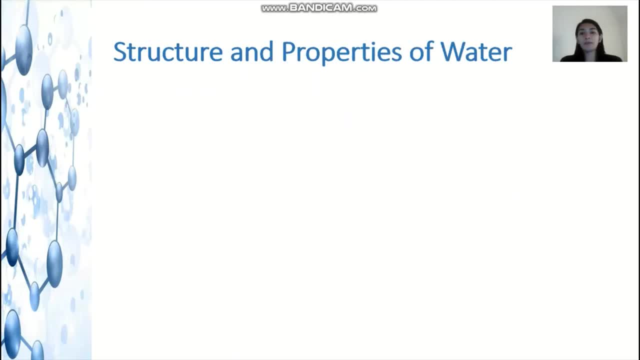 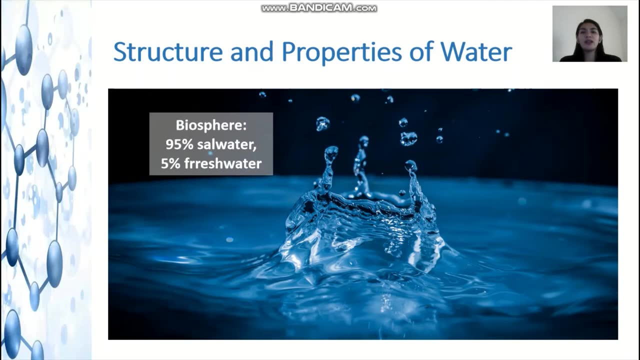 the opposite of your heat of vaporization. now, this have or let's discuss the structure and properties of water anyway, and I didn't know this already. okay, so you buy a sphere, it is actually 95% salt water and only 5% is fresh water. okay, so our bodies are actually 70% water and it is. 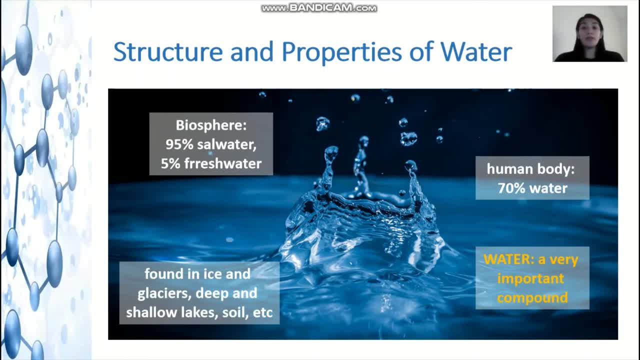 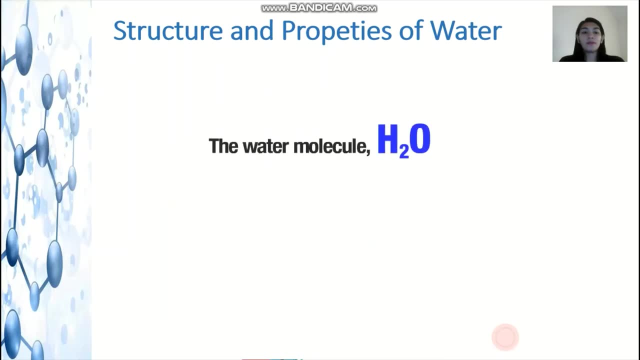 a very, very important compound. okay, so water break tile. here I have a glass of water and refreshing a water. no, so let's have a closer look at water using the short movie. so this is your weather molecule, our oxygen and hydrogen, with a spoiler ends: a slightly negative charged and a slightly positive charge. 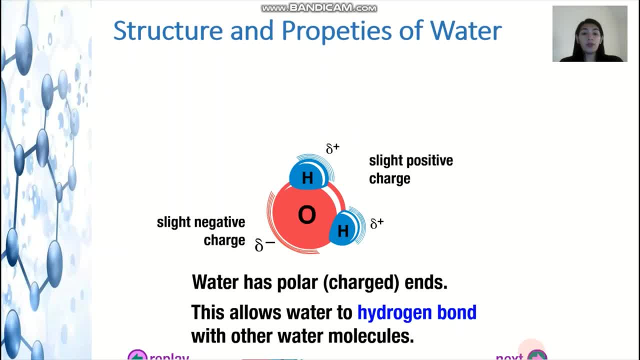 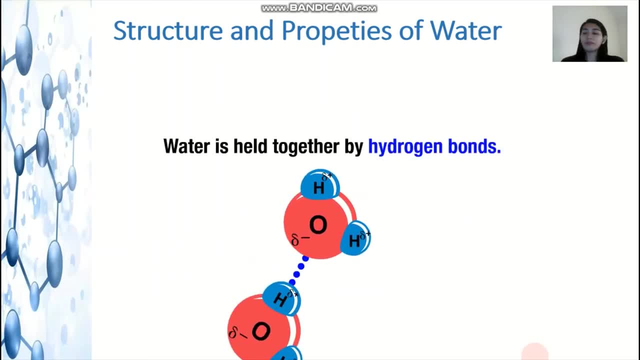 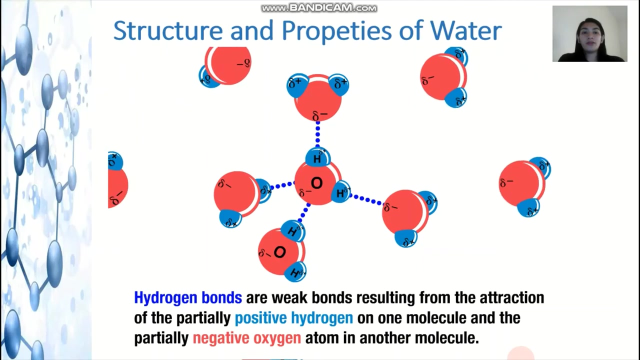 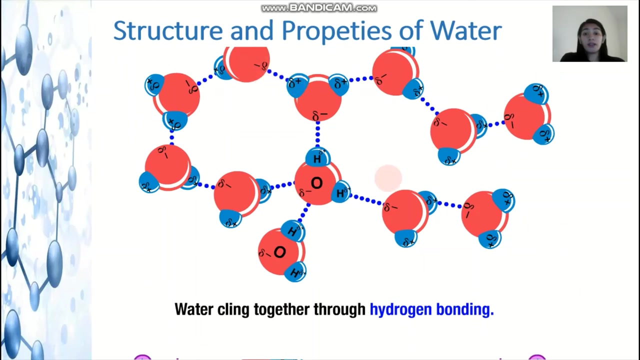 okay, so this would allow your water to hydrogen bond with other molecules. okay, this is what happens when the water molecule of me- but they are together behind- is advanced and okay, so you see the bonding. so hydrogen bonds are actually the weak bonds resulting from your bonding. okay, so the water clean together through. 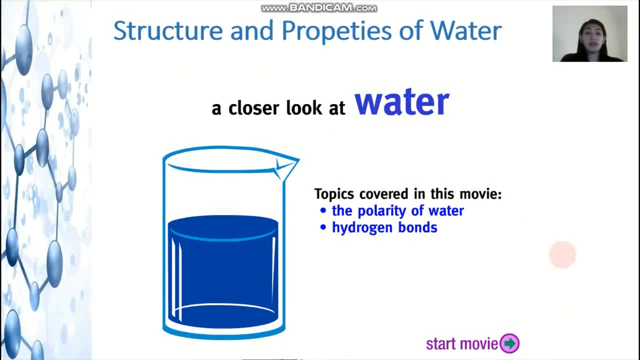 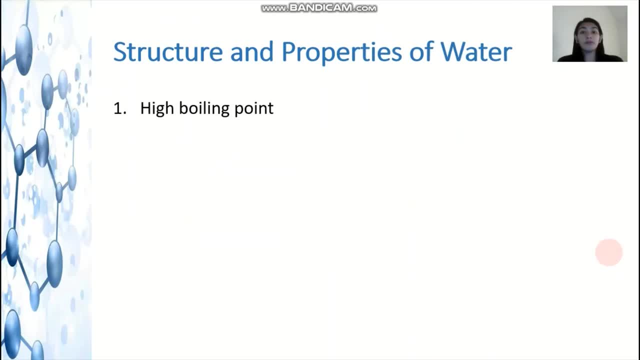 hydrogen bonding. okay, so that's all you can. you name bonding, compare, no, just a short animation. okay, now let's have. these are the properties of water, so we have high boiling point, high specific heat, high density in its liquid form, high heat of vaporization and high surface tension. now let's go to the types and 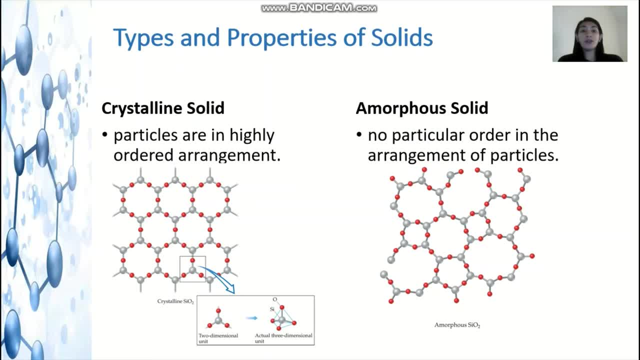 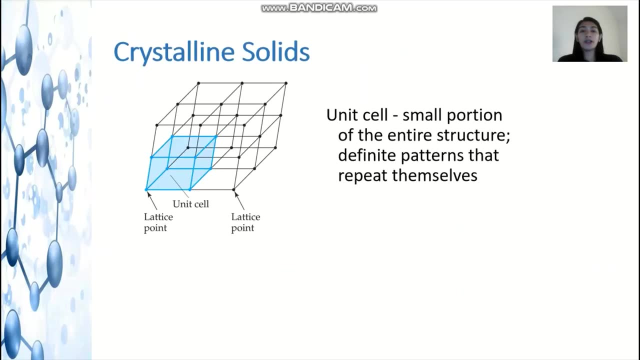 properties of solid. so we actually have two types: the crystalline solid and the amorphous solid. so for the crystalline solids, the particles are arranged in an orderly manner. for the amorphous solids, there's no particular order of arrangement of the particles. okay, so crystalline solids are arranged. 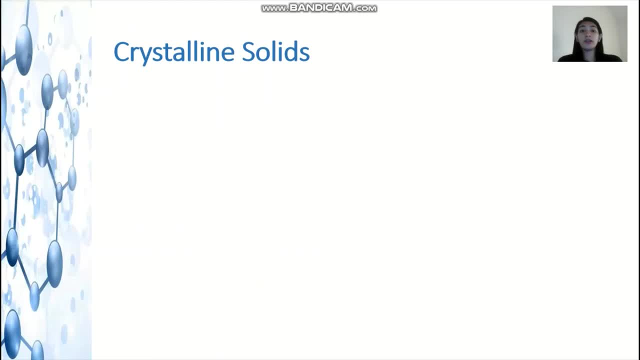 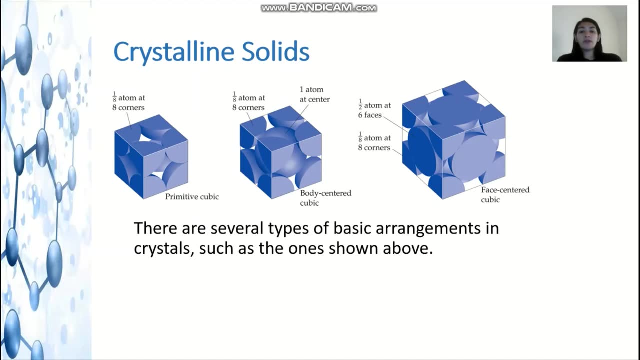 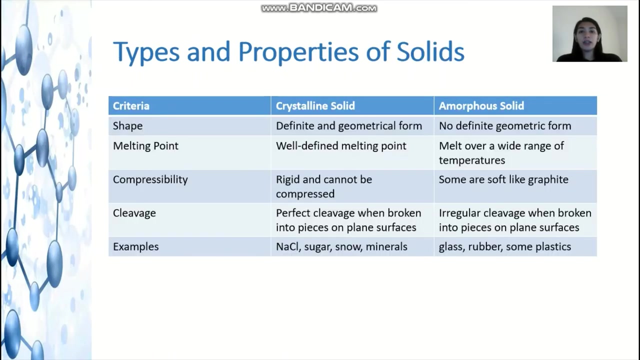 as a unit cells. there are patterns, so there are different types of unit cells according to their shape. so here are also the arrangements of your crystals. it can be primitive, body centered and face centered, cubic. okay, now these are the types and properties of solids. so according to shape, we defined it earlier. 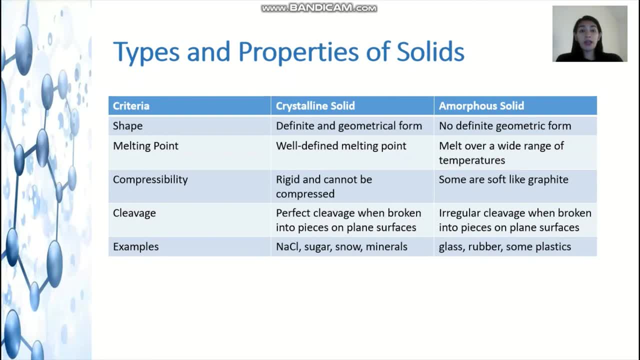 germina, we have a mass helping it in terms of volume. it's a definiteVERM in its comprising form. so, like I saidIVE can be possible used all kinds of fluids. soぁwe can prefer to have a product here which lets one hand be in the system of capabilities and one is a 21.25 % relationship. 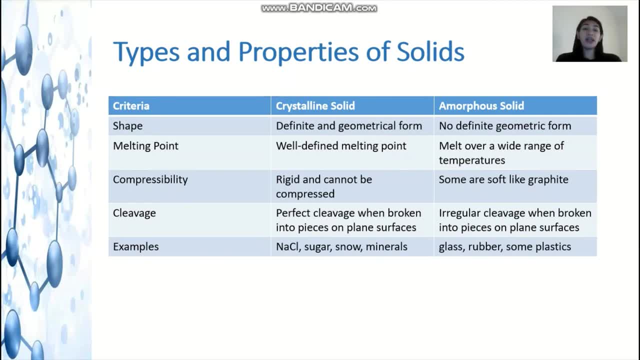 after is a recycler onto the fabric, connect to a close to the exact distance of the solid. solid. solid is it is irregular, okay, so cleavage is yung surface kapag nag break sya okay, or broken into pieces. so examples of crystalline solids are your salt, sugar, snow and minerals. amorphous solid. 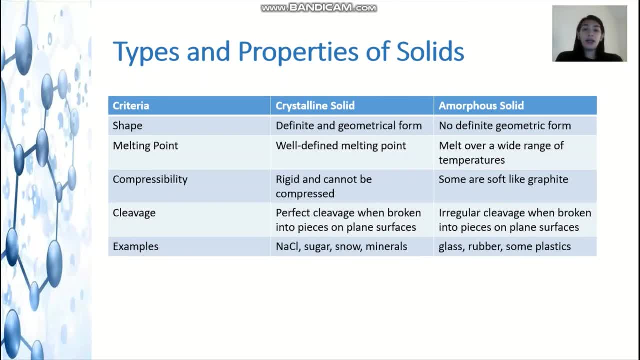 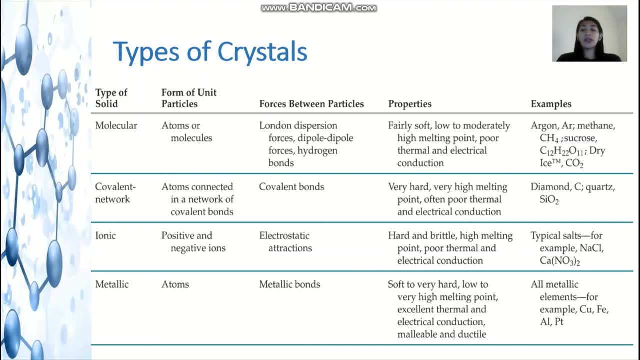 example is glass rubber and some of your plastics. okay, types of crystals: there are actually four types. you have the molecular covalent network, ionic and your metallic crystals. okay, so ang focus natin dito would be the forces between the particles. okay, so yung molecular crystals. 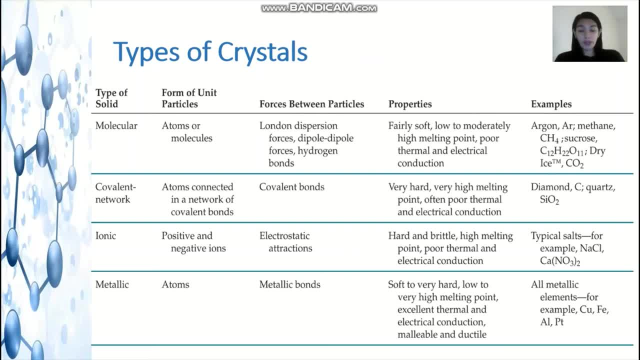 they have london dispersion forces, dipole dipole forces or hydrogen bonds, so they're fairly soft. you have low to moderately high melting point, so examples of these are methane, sucrose, dry ice and your carbon dioxide. for covalent crystals you also have um. it is held together by covalent. 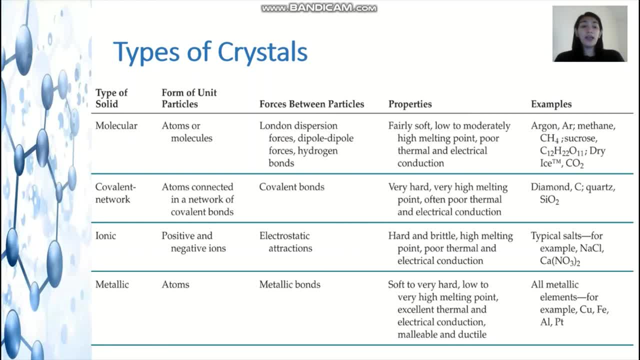 bonds, so they're very hard. they have very high melting point, and examples of these are your diamond and quartz. so for ionic crystals, they're held together by electrostatic attractions. they're hard and brittle, with high melting point. they have poor thermal and electrical conduction. so examples of these are your typical salts. and last you have your metallic crystals. 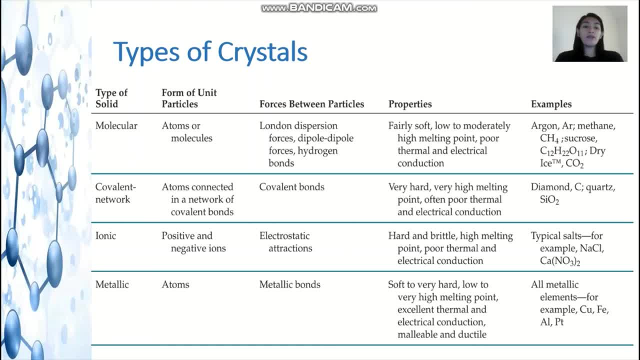 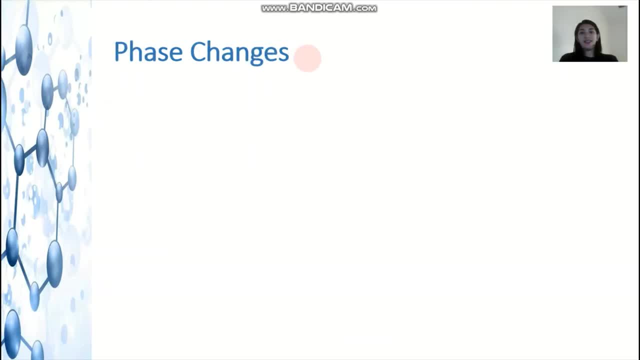 so they're held together by metallic bonds. so they're soft to very hard and they have low to very high melting point. so examples of these are all metallic elements. so next let's go to phase changes. so these are already discussed in your general chemistry one. so as you can see now this is just 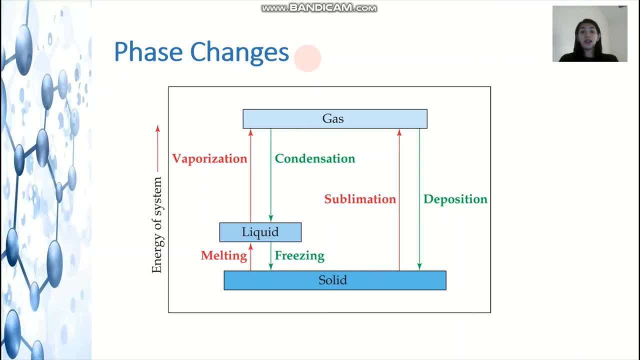 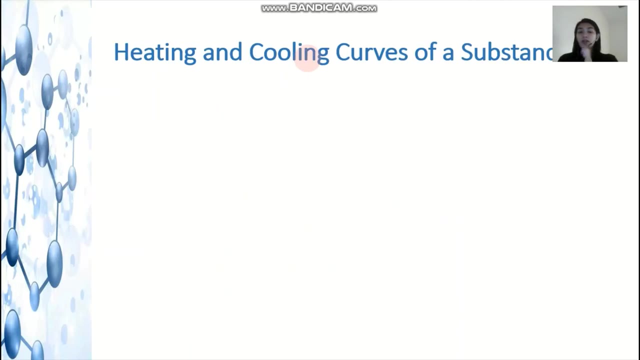 an easier diagram for you to visualize now, the changes happening from solid to liquid, liquid to gas and vice versa. okay, now the phase changes could also be observed in your heating and cooling curves of a substance. okay, so the phase changes could also be observed using your heating curve. 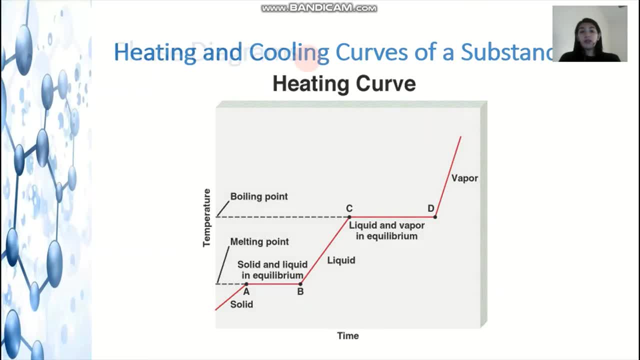 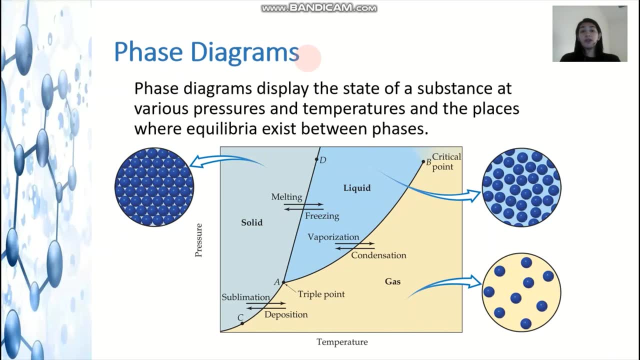 your those that will be shown over between an answer block and this is specifically 回…". yeah right, they were dominate. did not use the 12 B�Su. so the point jestem cl��, period zero in equilibrium. So in this phase diagram let's see now the AB line. So this is the liquid vapor. 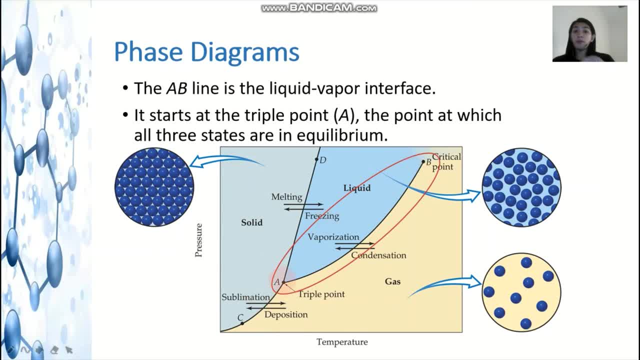 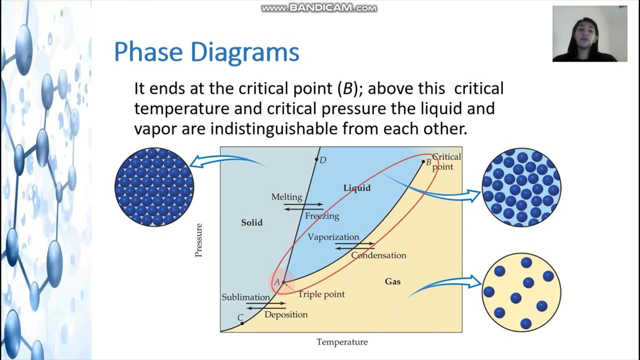 interface. So it starts at this point, at the triple point. So it is the point at which all three states are in equilibrium. okay, So it ends at the critical point B. above this critical temperature and critical pressure, The liquid and the vapor are indistinguishable from each other. 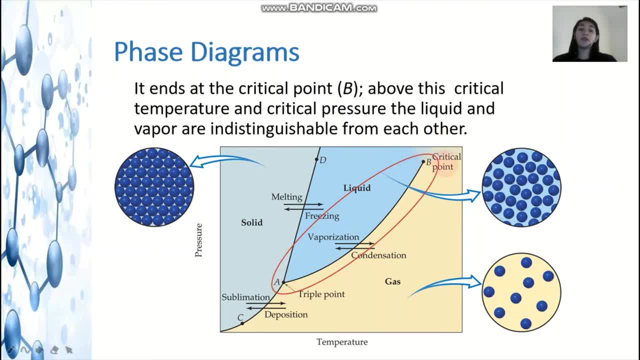 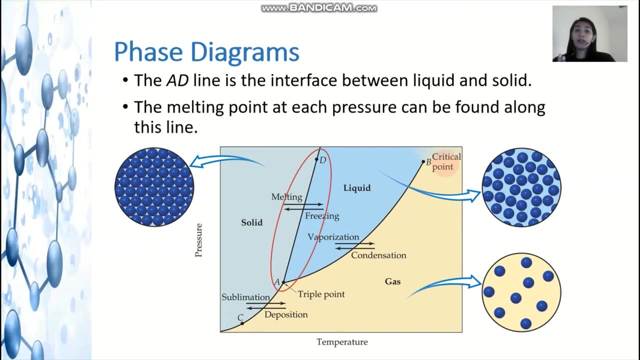 So pag lumapas na dito, hindi na natin ma-identify kung liquid ba siya or gas. okay, So each point along this line is the boiling point of the substance at that pressure. So next we have the AD line. So this is the interface between the liquid and solid. okay, So the melting point at 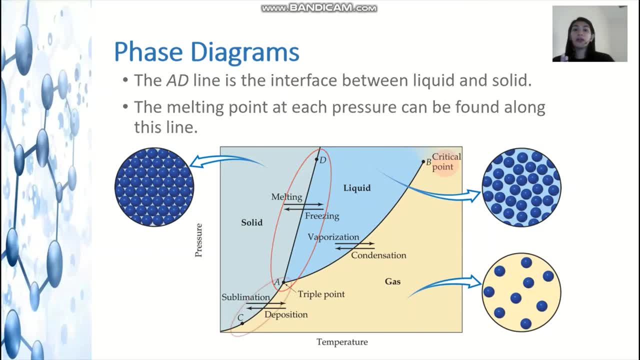 each pressure can be found along this line. okay, So next, so below the A, the substance cannot exist in the liquid state, So it could actually exist only as gas. Okay, So along the AC line the solid and gas phases are in equilibrium. So this is the.